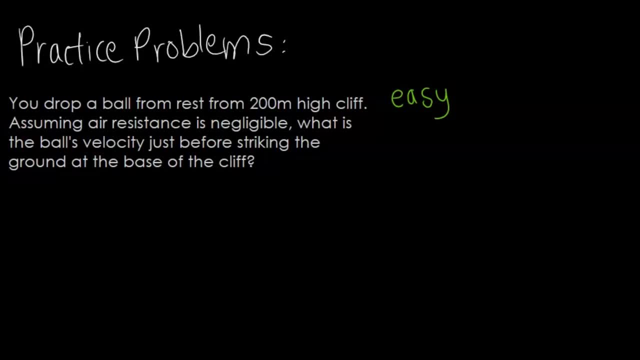 All right. so this is a video supplement to the AP Physics 1 exam review for kinematics. So if you guys haven't seen that video, I would recommend checking that out after trying to solve this problem. So yeah, let's just get right into it. So you drop a ball from rest, from 200 meter. 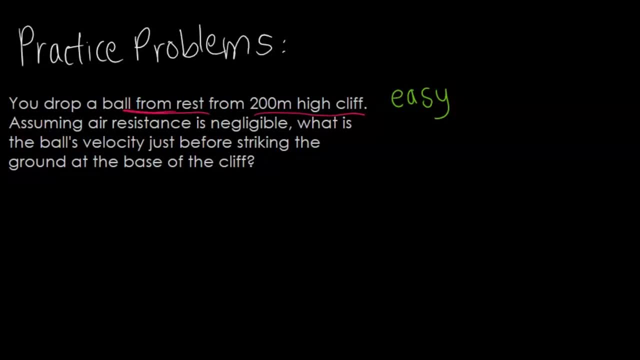 high cliff. So the ball is dropped from rest. Assuming air resistance is negligible, what is the ball's velocity just before striking the ground at the base of the cliff? So let's write out our known variables, which is a strategy we want to use for kinematics. So the first thing. 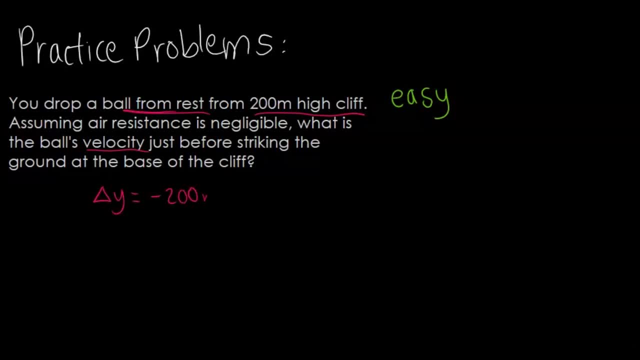 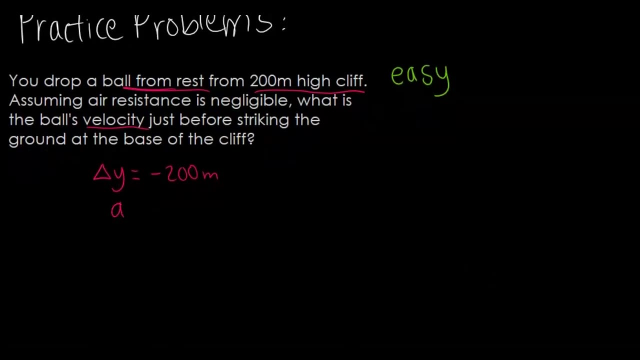 that I know is that the Y displacement is going to be negative 200 meters. That's because we identified the top of the cliff, the top of the 200 meters, as the zero point line. So if you drop something below that 200 meters, that's going to be the negative. The next thing that I want to 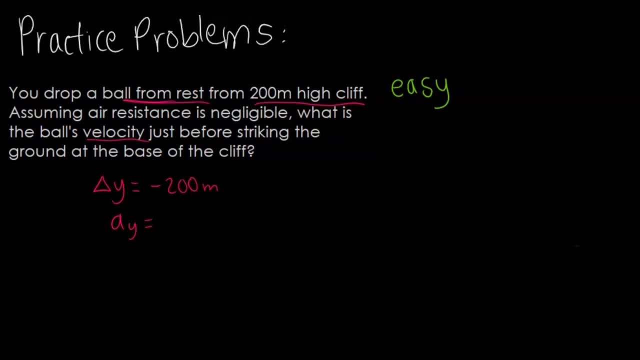 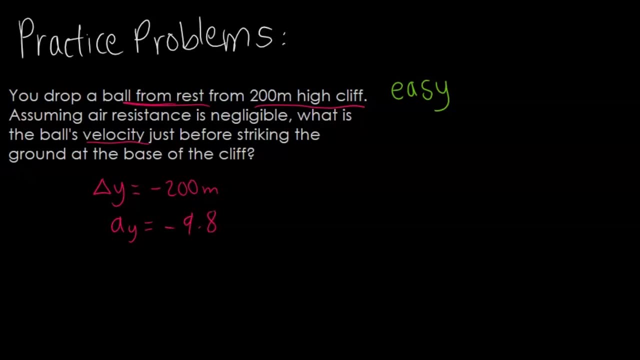 take note of is the acceleration in the Y direction And since this is a ball we're just dropping from rest from a cliff, it's going to be in freeway And any object in freefall on Earth is going to experience a gravitational constant of negative. 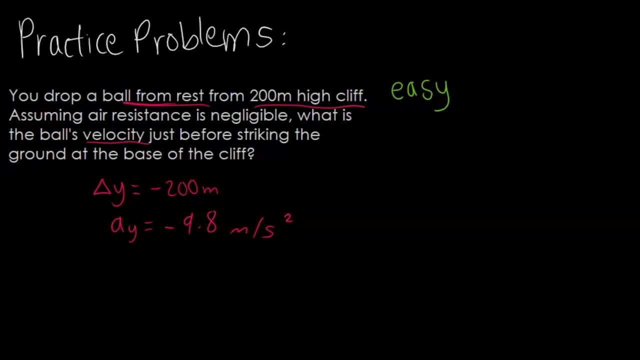 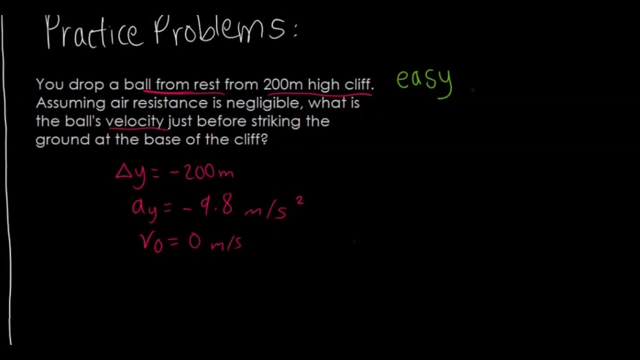 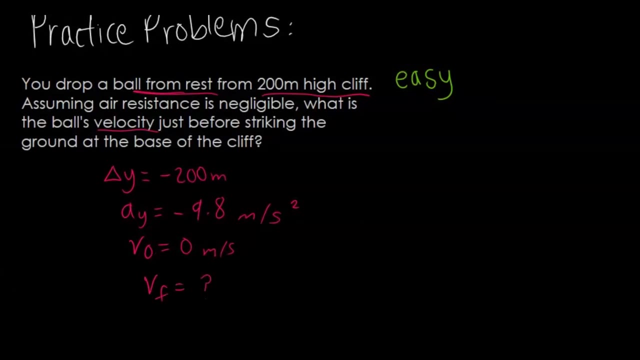 9.8 meters per second squared. Another thing is it's dropped from rest, So the initial velocity is just going to be zero meters per second, And we want to find the ball's velocity just before striking the ground. So that is what we're going to be solving for the final velocity. Now, if you, 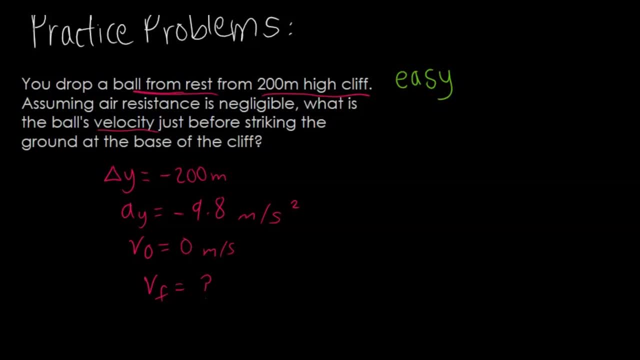 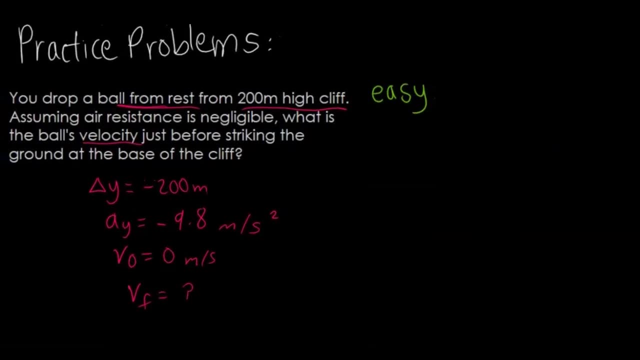 think about it. the final velocity is zero right when it hits the ground. That's technically the final velocity, But for our case we want to find the velocity just before striking the ground. All right, so let's pick out one of our equations that has these three known variables and can help. 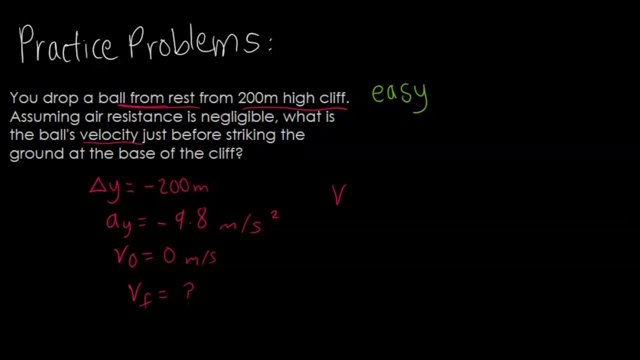 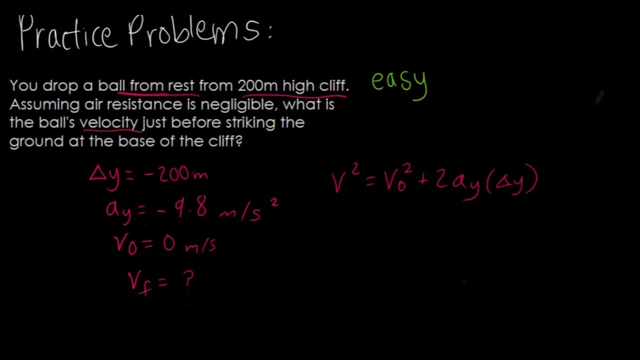 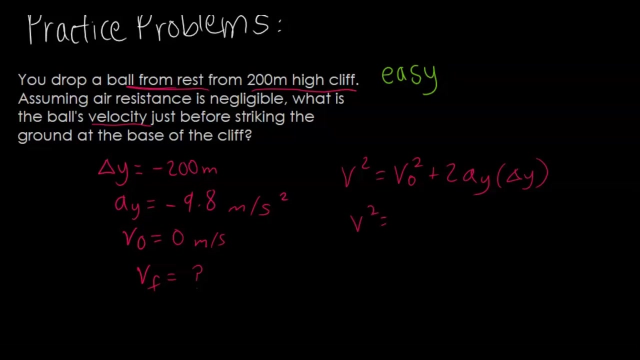 us find the final variable, And that equation is going to be: velocity squared, final velocity squared, initial velocity squared plus two times the acceleration in the Y direction, And then our displacement, or just Y. So yeah, now let's just plug in our numbers. So our V squared is just going to be: